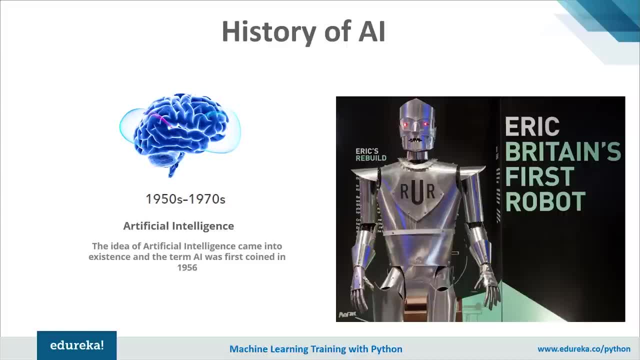 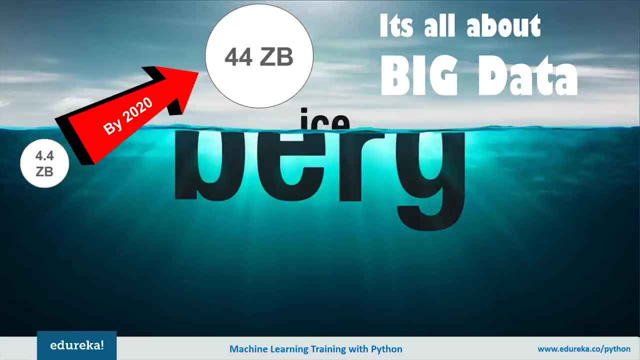 very small amount of data. The data we had was not enough to predict the accurate result, But now there's a tremendous increase in the amount of data. statistics suggest that by 2020, the accumulated volume of data will increase from 4.4 zettabytes to roughly around 44 zettabytes. 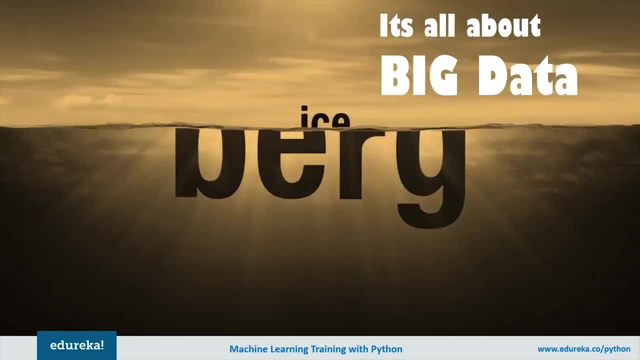 or 44 trillion GBs of data. along with such enormous amount of data, Now we have more advanced algorithm and high-end computing power and storage that can deal with such large amount of data. As a result, it is expected that 70% of Enterprise will implement AI over the next 12 months. 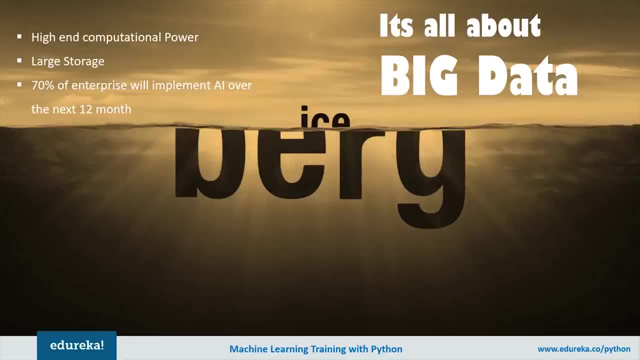 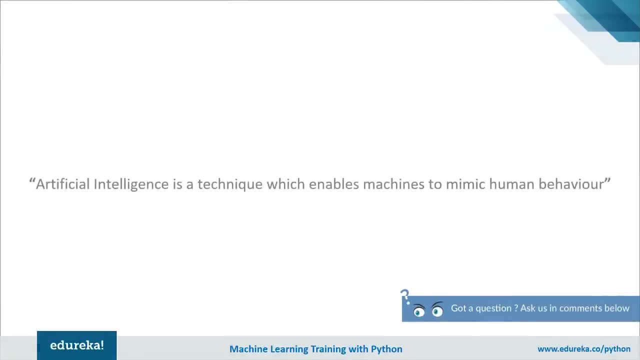 which is up from 40% in 2016 and 51% in 2017. just for your understanding, What is AI? Well, it's nothing but a technique that enables the machine to act like humans by replicating the behavior and nature. with AI, 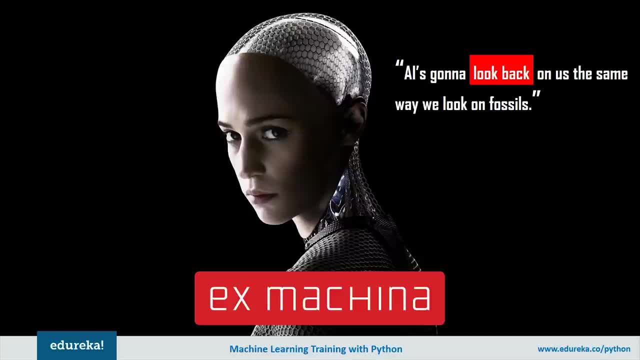 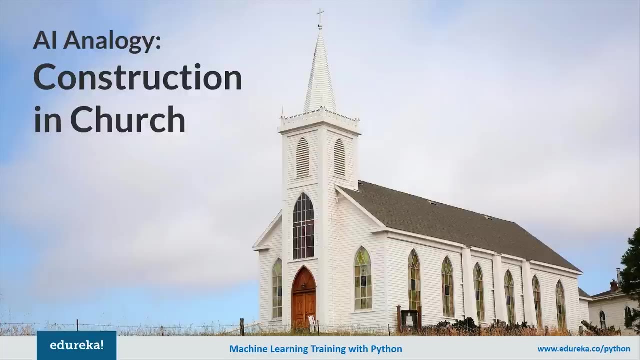 It is possible for machine to learn from the experience. the machines adjust their responses based on new input, Thereby Information like tasks. artificial intelligence can be trained to accomplish specific tasks by processing large amount of data and recognizing pattern in them. You can consider that building an artificial intelligence is like building a church. 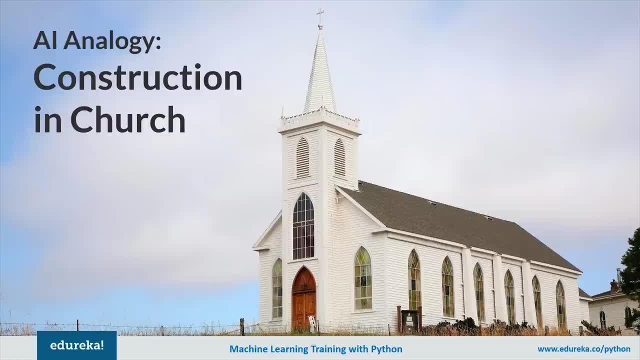 The first church took generations to finish, So most of the workers were working in it never saw the final outcome. those working on it took pride in their crafts: building bricks and chiseling stone that was going to be placed into the great structure So as AI researchers. 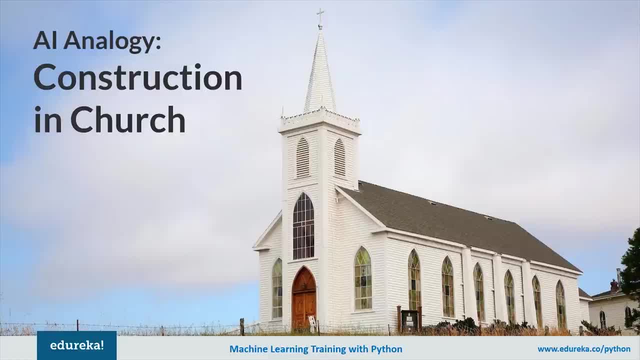 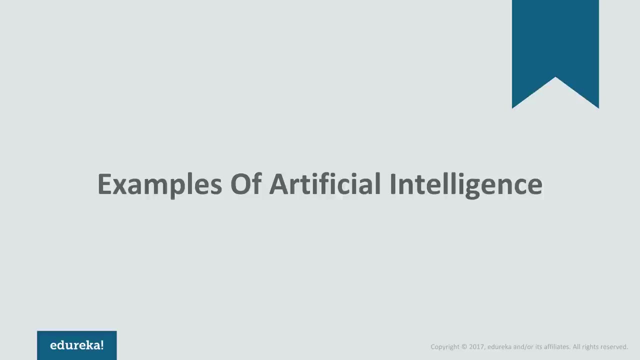 We should think of ourselves as humble brickmakers whose job is to study how to build components, example passes, planners or learning algorithm, or except anything that someday someone and somewhere will integrate into the intelligent systems. some of the examples of artificial intelligence from our day-to-day life are Apple series just playing computer, Tesla self-driving. 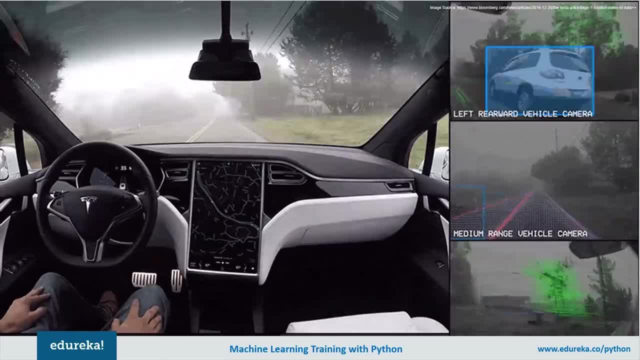 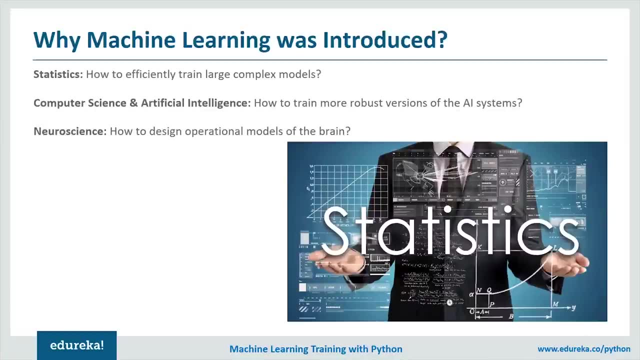 car and many more. these examples are based on deep learning and natural language processing. Well, this was about what is AI And how it gains its high. so, moving on ahead, let's discuss about machine learning and see what it is and why it was even introduced. well, machine learning came into existence. 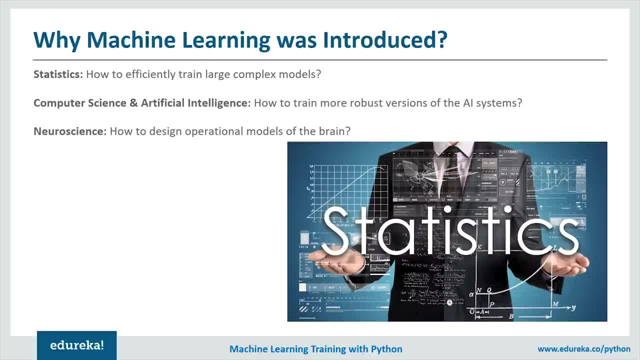 in the late 80s and the early 90s. But what were the issues with the people which made the machine learning come into existence? Let us discuss them one by one. in the field of statistics, The problem was how to efficiently train large, complex model. in the field of computer science, 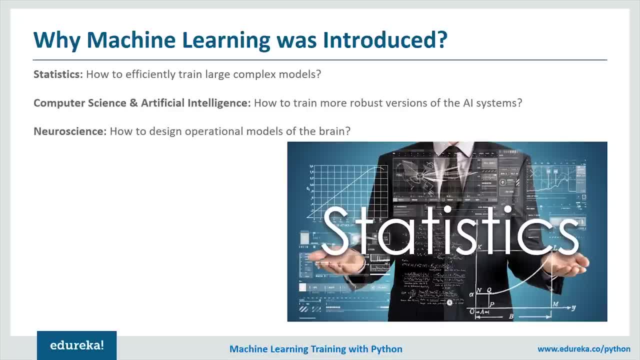 and artificial intelligence, The problem was how to train more robots. The problem was version of AI system, while in the case of neuroscience, problem faced by the researchers was how to design operational model of the brain. So these were some of the issues which had the largest influence and led to the existence. 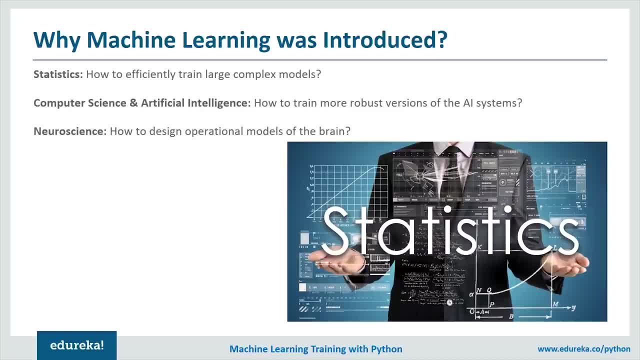 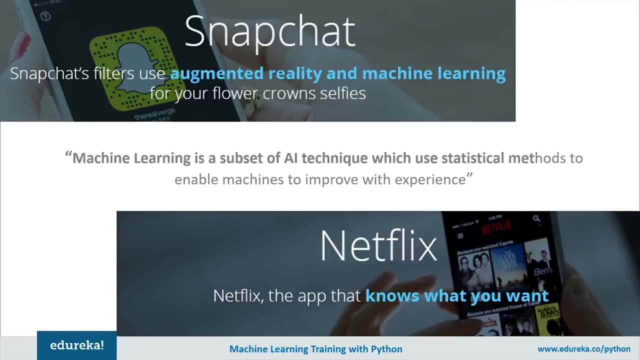 of the machine learning. now, this machine learning shifted its focus from the symbolic approaches It had inherited from the AI and move towards the methods and model It had bought from statistics and probability theory. So let's proceed and see what exactly is machine learning. well, machine learning is a system. 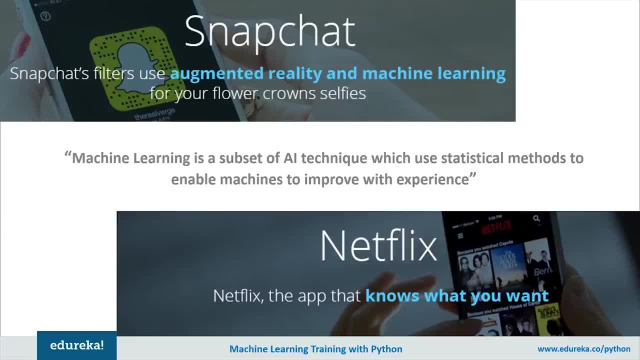 a subset of AI which enables the computer to act and make data-driven decisions to carry out a certain task. these programs or algorithms are designed in a way that they can learn and improve over time when exposed to new data. Let's see an example of machine learning. 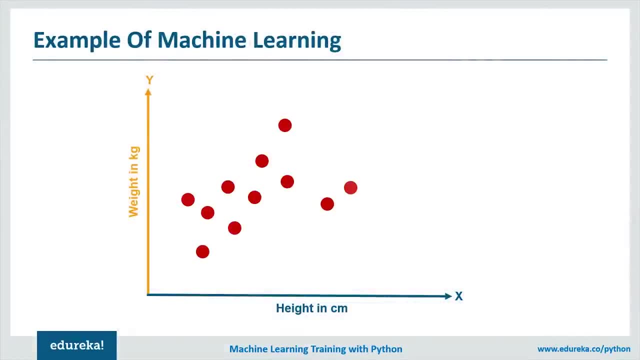 Let's say you want to create a system which tells the expected weight of a person based on its height. The first thing you do is you collect the data. Let's see. This is how your data looks like now. each point of the graph represent one data point. 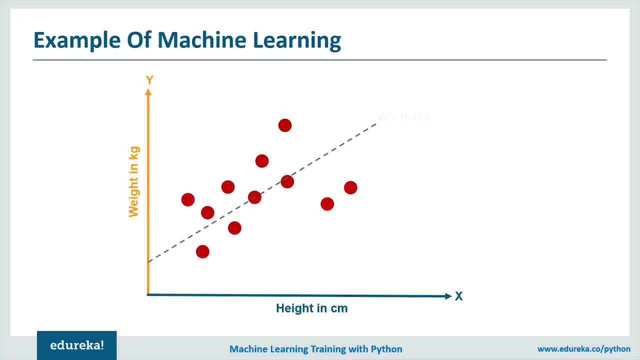 to start with, We can draw a simple line to predict the weight based on the height. For example, a simple line: W equal H minus 100, where W is weight in kgs and edges height in centimeter. This line can help us to make the prediction. 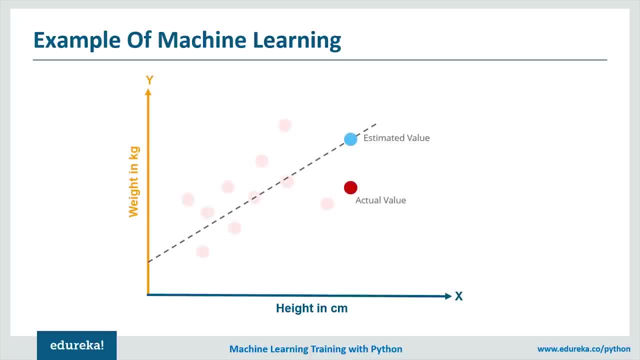 Our main goal is to reduce the difference between the estimated value and the actual value. So, in order to achieve it, we try to draw a straight line that fits through all these different points and minimize the error. So our main goal is to minimize the error and make them as small as possible. 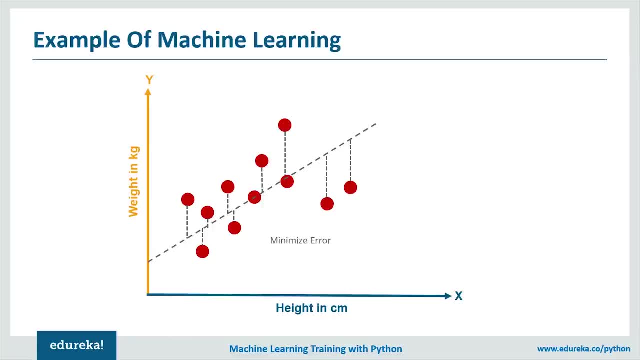 Decreasing the error or the difference between the actual value and estimated value increases the performance of the model further on. the more data points we collect, the better our model will become. we can also improve our model by adding more variables and creating different prediction lines for them once the line is created. 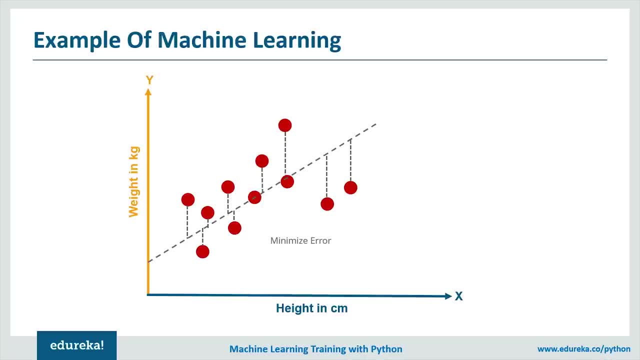 So from the next time, if we feed a new data, for example height of a person, to the model, it would easily predict the data for you and it will tell you what is predicted weight could be. I hope you got a clear understanding of machine learning. 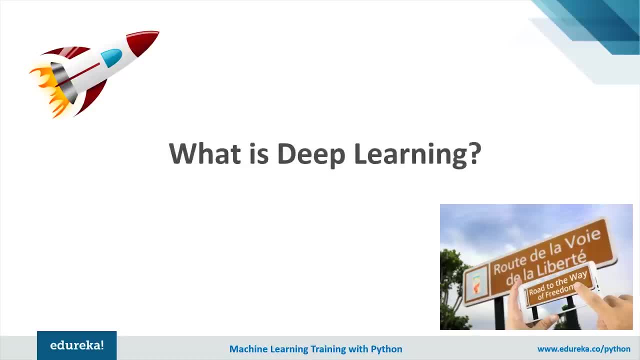 So, moving on ahead, let's learn about deep learning. Now, what is deep learning? You can consider deep learning model as a rocket engine, and its fuel is its huge amount of data that we feed to these algorithms. The concept of deep learning is not new, but recently its hype has increased. and deep learning 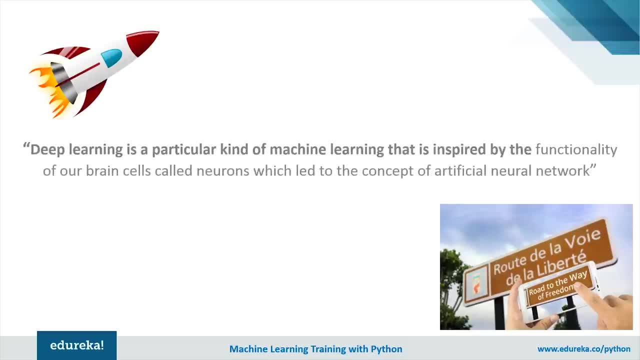 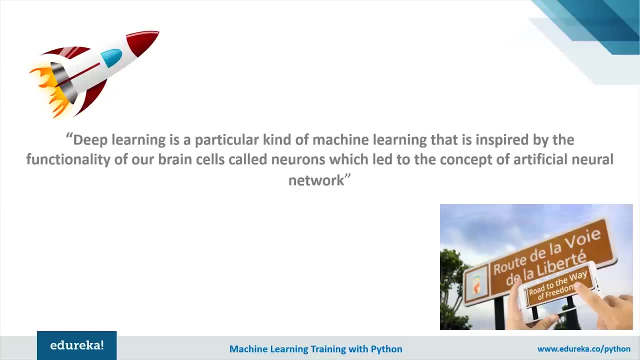 is getting more attention. This field is a particular kind of machine learning that is inspired by the functionality of our brain cells called neuron, which led to the concept of artificial neural network. It simply takes the data Distraction between all the artificial neurons and adjust them according to the data pattern. 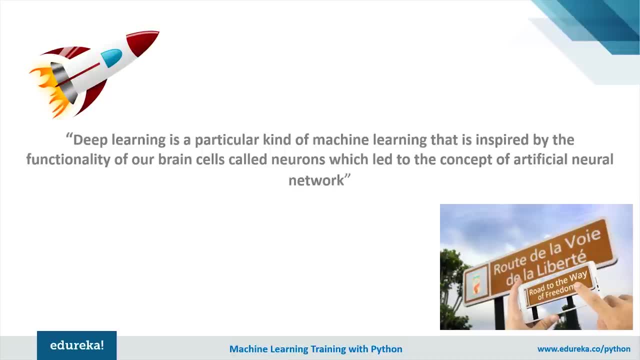 more neurons are added at, the size of the data is large, it automatically features learning at multiple levels of abstraction, thereby allowing a system to learn complex function mapping without depending on any specific algorithm. You know what? No one actually knows what happens inside a neural network and why it works so well. 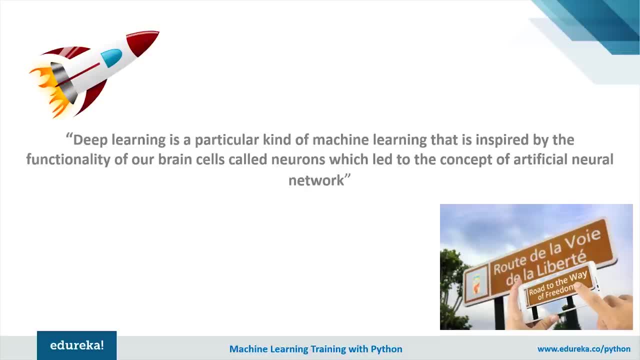 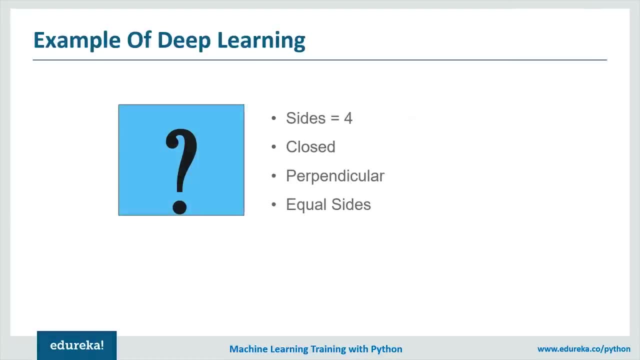 So currently you can call it as a black box. Let us discuss some of the example of deep learning and understand it in a better way. Let me start with a simple example and explain you how things happen at a conceptual level. Let us try and understand how you recognize a square from other shapes. 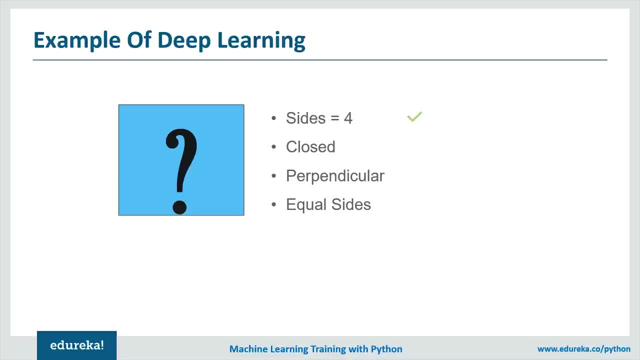 The first thing you do is you check whether there are four lines associated with the figure or not. simple concept, right. if yes, we further check if they are connected and closed, again if yes. we finally check whether it is perpendicular and all its sides are equal. correct, if everything. 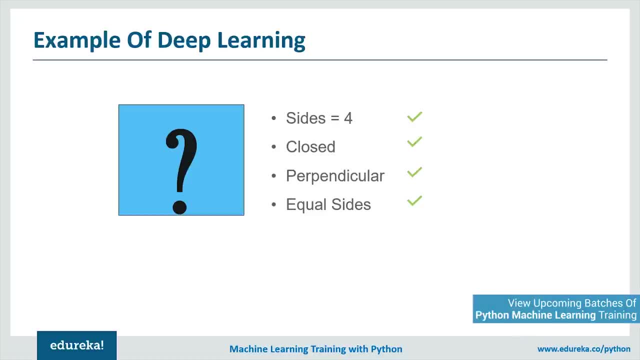 fulfills. Yes, Well, it is nothing but a nested hierarchy of concepts. what we did here? We took a complex task of identifying a square, in this case, and broke it into simpler task. Now this deep learning also does the same thing, but at a larger scale. let's take an. 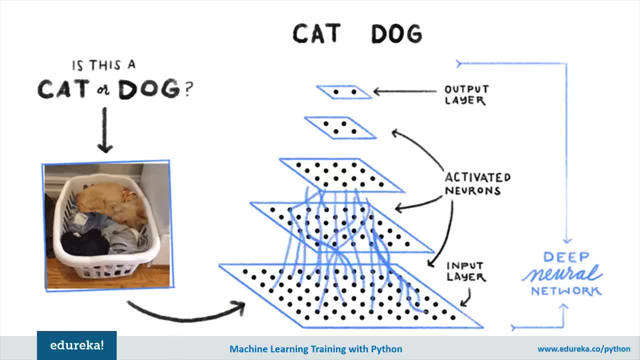 example of machine which recognizes the animal. the task of the machine is to recognize whether the given image is of a cat or of a dog. What if we were asked to resolve the same issue using the concept of machine learning? what we would do? first, We would define the features, such as check whether the animal has whiskers or not, or 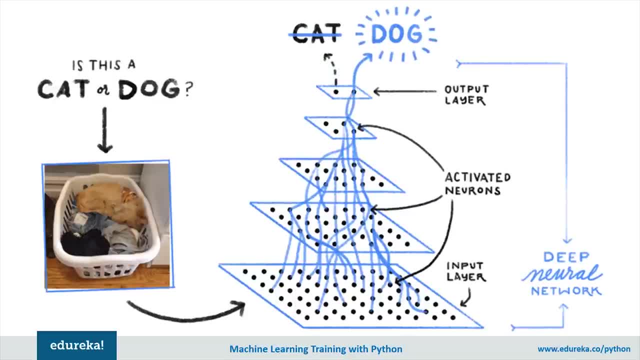 check if the animal has pointed ears or not, or whether its tail is straight or curved. in short, we will define the facial features and let the system identify which features are more important in classifying a particular animal. now, when it comes to deep learning, it takes this to one step ahead. deep learning automatically finds out the feature which. 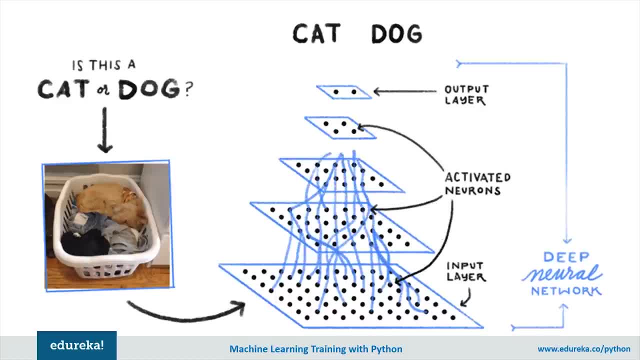 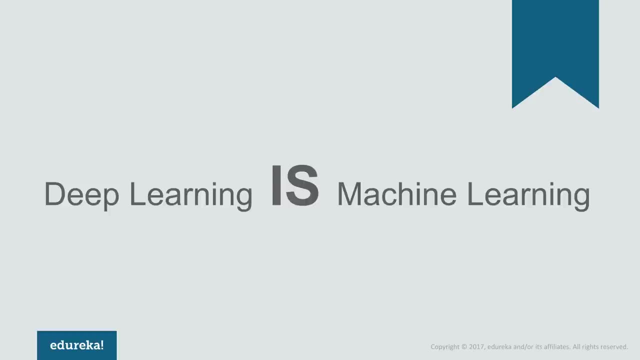 are most important for classification, compared to machine learning, where we had to manually give out that features. by now I guess you have understood that AI is a bigger picture and machine learning and deep learning are its subpart, So let's move on and focus our discussion on machine learning and deep learning. the 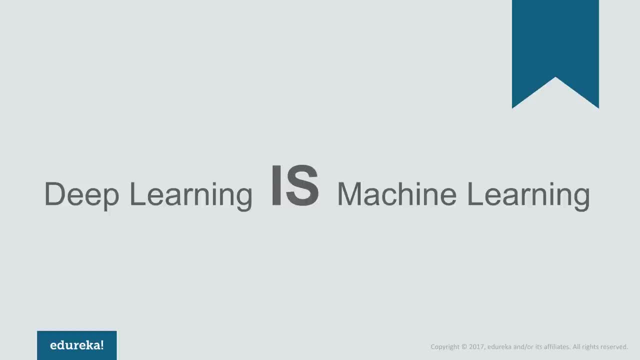 easiest way to understand the difference between the machine learning and deep learning is to know that deep learning is machine learning. more specifically, It is the next evolution of machine learning. Let's take few important parameter and compare machine learning with deep learning. So, starting with data dependencies. 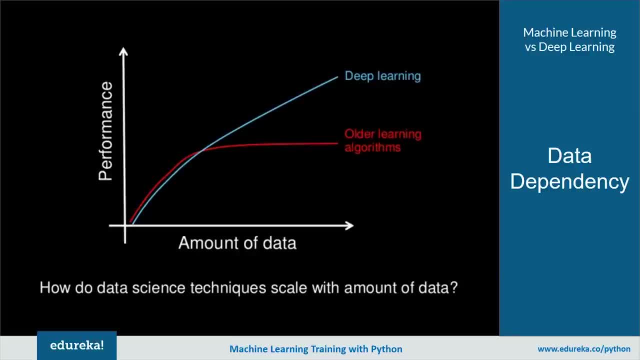 The most important Difference between deep learning and machine learning is its performance, as the volume of the data gets increased. from the below graph, You can see that when the size of the data is small, deep learning algorithm doesn't perform that well. but why? well, this is because deep learning algorithm needs a large amount of 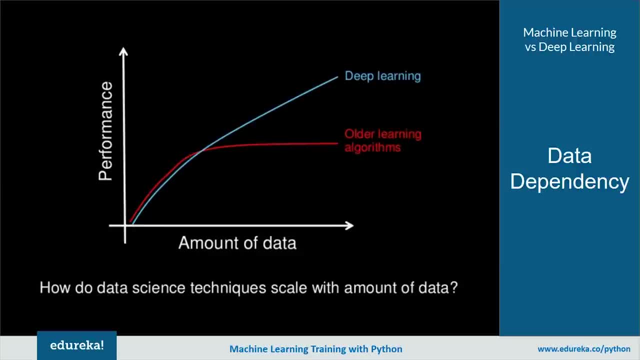 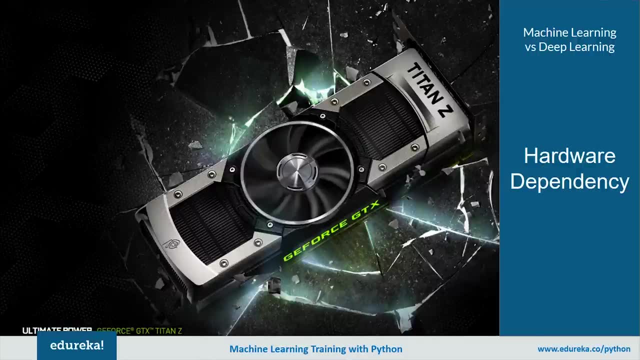 data to understand it perfectly. on the other hand, the machine learning algorithm can easily work with smaller data set fine. next comes the hardware dependencies. deep learning algorithms are heavily Dependent on high-end machines, while the machine learning algorithm can work on low-end machines as well. 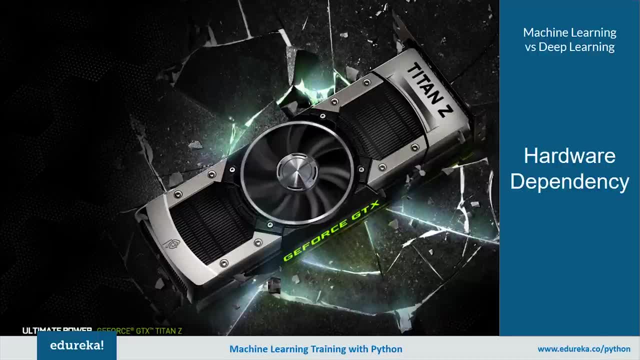 This is because the requirement of deep learning algorithm include GPUs, which is an integral part of its working. the deep learning algorithm required GPUs, as they do a large amount of matrix multiplication operations, and these operations can only be efficiently optimized using a GPU as it is built for this purpose only. our third parameter will be feature engineering. 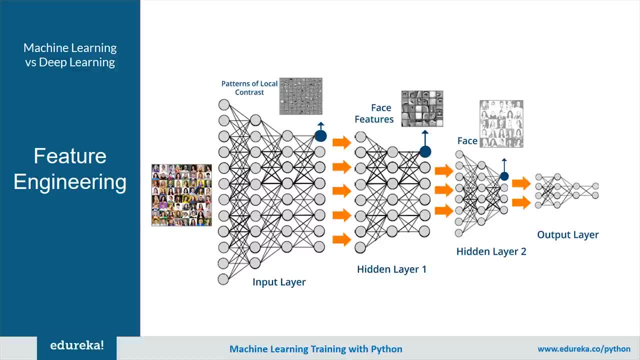 Well. feature engineering is a process of putting the domain knowledge to reduce the complexity of the data and make patterns more visible to learning algorithms. This process is difficult and expensive in terms of time and expertise. in case of machine learning, Most of the features are needed to be identified by an expert and then hand-coded as per the. 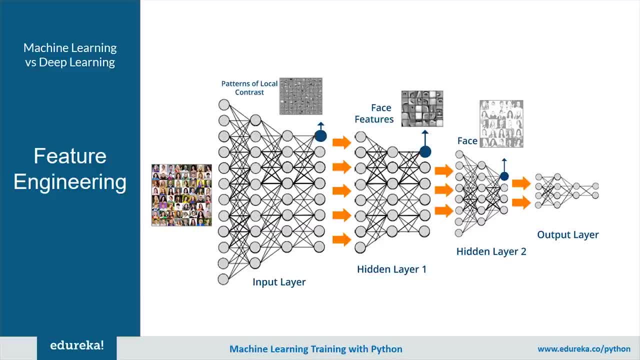 domain and the data type. for example, the features can be a pixel value, shapes, texture, position, orientation or anything fine. The performance of most of the machine learning algorithm depends on how accurately the features are identified and extracted, whereas in case of deep learning algorithms, It try to learn high-level features from the data. 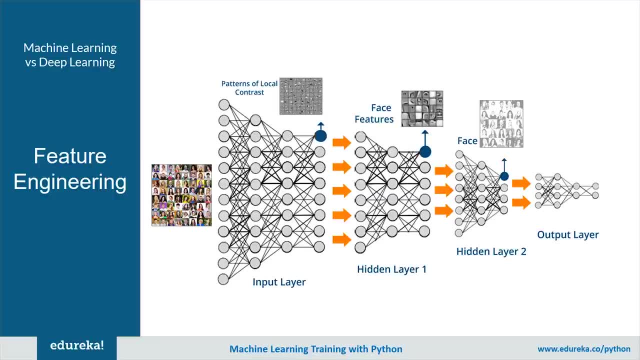 This is a very distinctive part of deep learning which makes it way ahead of traditional machine learning. deep learning reduces the task of developing new feature extractor for every problem. like in the case of CNN algorithm, It first try to learn the low-level features of the image, such as edges and lines, and then 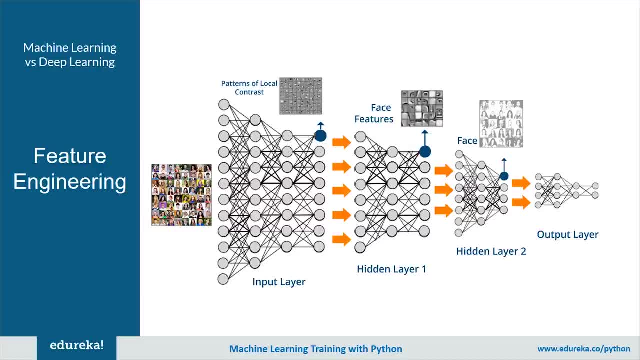 it proceeds to the parts of faces of people and then finally to the high-level representation of the face. I hope the things are getting clear to you. So let's move on ahead and see the next parameter. So our next parameter is problem-solving approach. when we are solving a problem using traditional 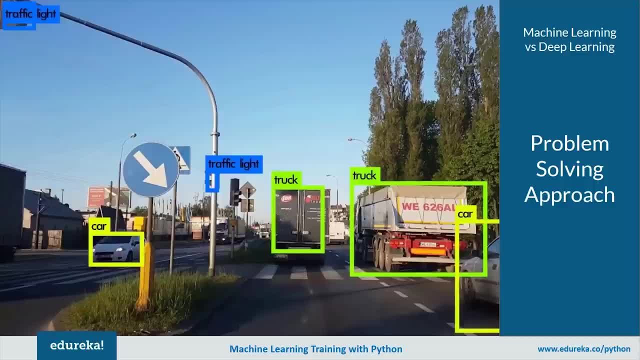 machine learning algorithm. It is generally recommended that we first break down the problem into different sub parts, solve them individually and then finally combine them to get the desired result. This is how the machine learning algorithm Handles the problem. on the other hand, the deep learning algorithm solves the problem. 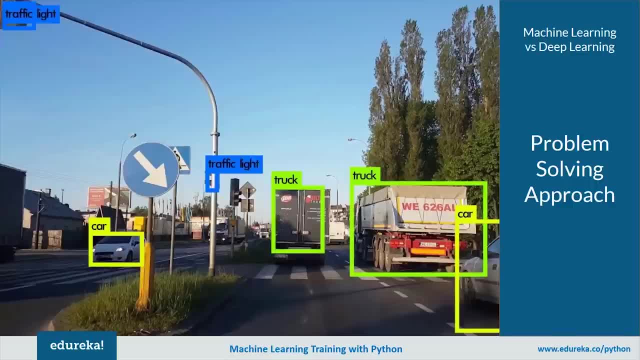 from end to end. Let's take an example to understand this. suppose you have a task of multiple object detection and your task is to identify what is the object and where it is present in the image. So let's see and compare. how will you tackle this issue using the concept of machine learning? 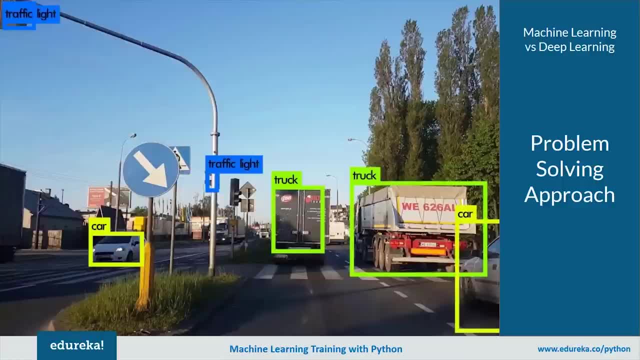 and deep learning, starting with machine learning. in a typical machine learning approach, You would first divide the problem into two step: first object detection and then object organization. first of all, you would use a bounding box detection algorithm like grab-cut, for example, to scan through the image and find out all the possible objects. 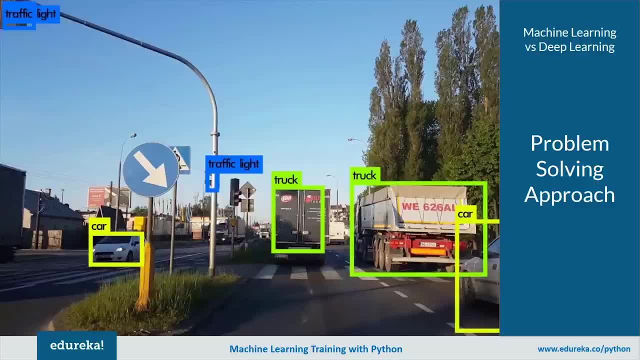 Now, once the objects are recognized, you would use object organization algorithm like SVM with hog to recognize relevant objects. Now, finally, when you combine the result, you would be able to identify what is the object and where it is present in the image. on the other hand, in deep learning approach, 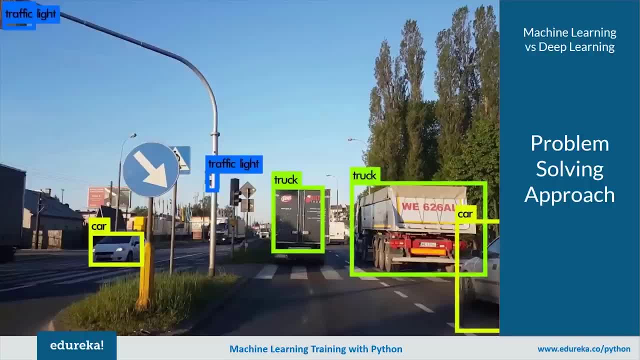 You would do the process from end to end, for example, in a Yolo net, which is a type of deep learning algorithm. you would pass an image and it would give out the location along with the name of the object. Now let's move on to a fifth comparison parameter: its execution time. 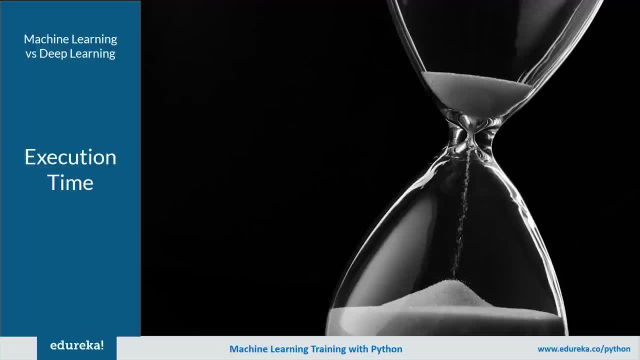 Usually a deep learning algorithm takes a long time to train. this because there's so many parameter in a deep learning algorithm that makes the training longer than usual. the training might even last for two weeks, or more than that If you are training completely from the scratch, whereas in the case 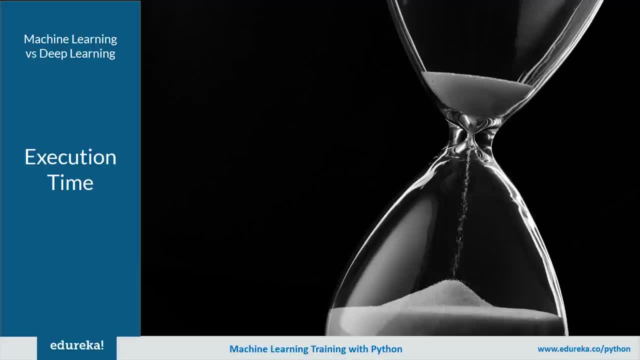 of machine learning. it relatively takes much less time to train, ranging from a few weeks to few hours. Now the execution time is completely reverse when it comes to the testing of data. during testing, the deep learning algorithm takes much less time to run, Whereas if you compare it with a Canon algorithm, 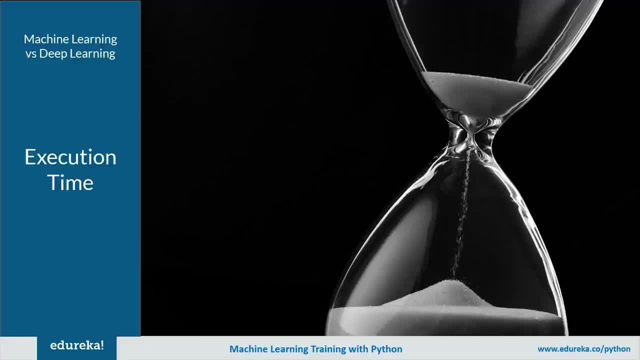 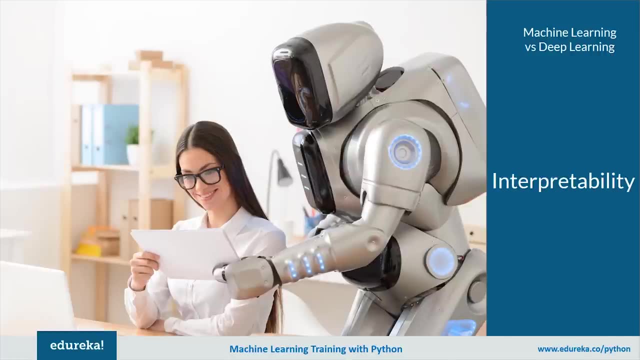 which is a type of machine learning algorithm. the test time increases as the size of the data increase. last but not the least, We have interpret ability as a factor for comparison of machine learning and deep learning. This factor is the main reason why deep learning is still taught. 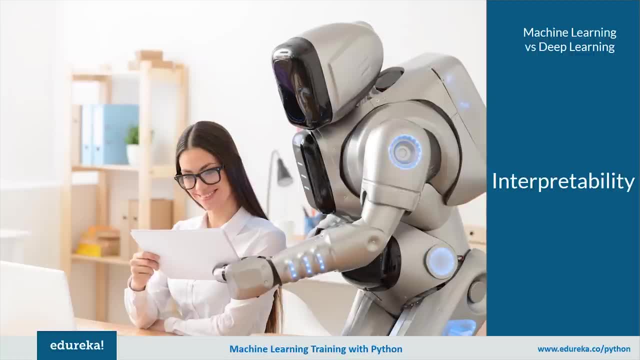 10 times before anyone uses it in the industry. Let's take an example. Suppose we use deep learning to give automated scoring to essays. the performance it gives in scoring is quite excellent and is near to the human performance, but there's an issue with it. 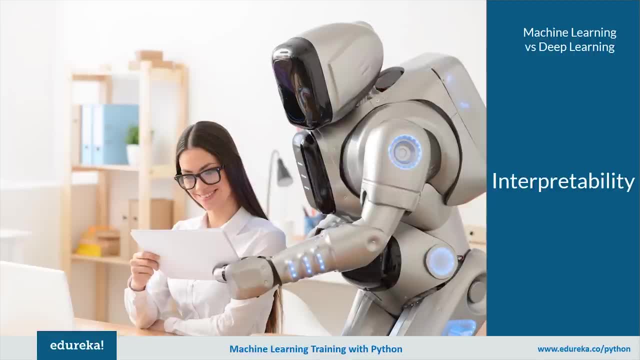 It does not reveal why it has given that score. indeed, mathematically, It is possible to find out that which node of a deep neural network was activated, but we don't know what the neurons are supposed to model and what these layers of neuron were doing collectively. 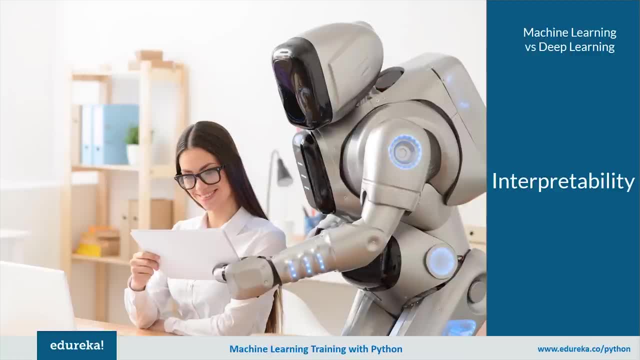 So he failed to interpret the result. on the other hand, machine learning algorithm like decision tree gives us a crisp rule for why it chose and what it chose, So it is particularly easy to interpret the reasoning behind it. Therefore, the algorithms like decision tree and linear or logistic regression are primarily used. 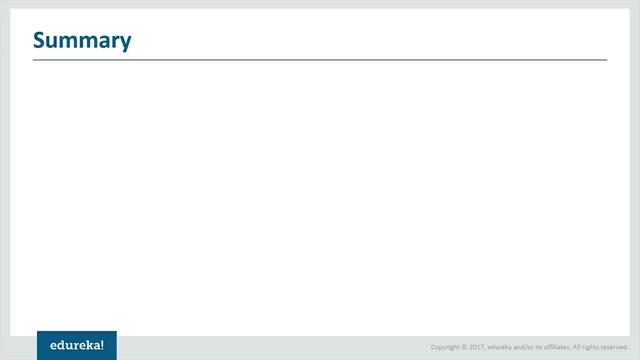 in industry for interpret ability. before we end this session, Let me summarize. Thanks for you. machine learning uses algorithm to parse the data, learn from the data and make informed decision based on what it has learned. fine, Now this deep learning structures algorithms and layers to create artificial neural network.